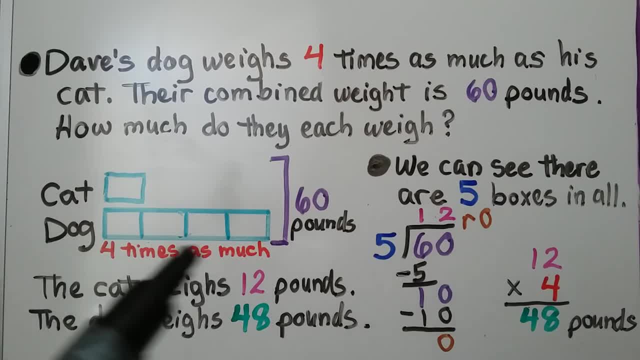 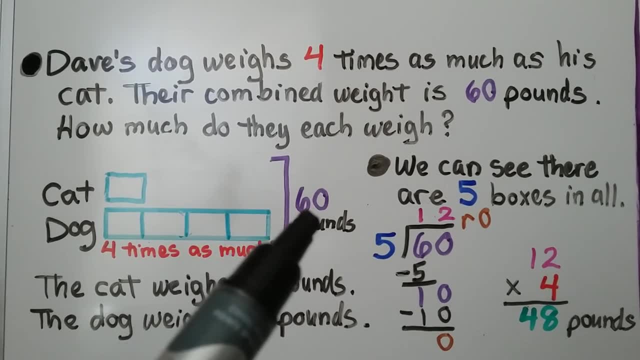 for the cat and the dog is four times as much. so we draw four boxes for the dog and their combined weight is 60 pounds and we put a bracket here with 60 for the 60 pounds We can see there are five boxes in all: 1,, 2,, 3,, 4, 5.. So we're going to divide 60 by 5.. 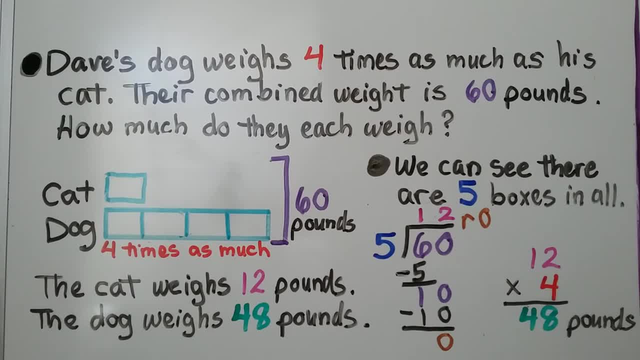 We can see: 60 divided by 5 is 12. that means the cat weighs 12 pounds. This one box is 12.. If the dog is 4 times as much, we do 12 times 4, which is 48.. The dog weighs 48 pounds. 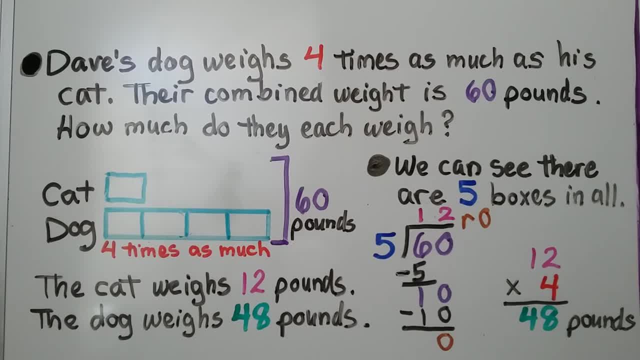 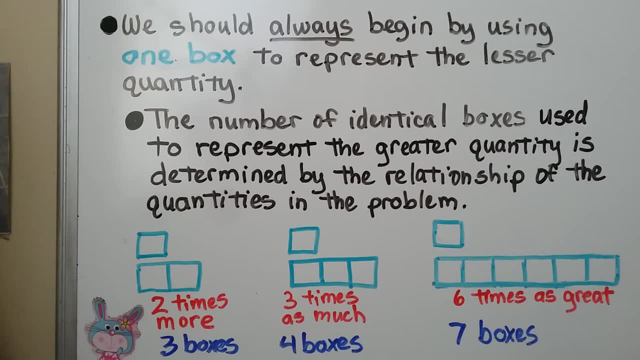 So let's talk about division, about this some more. We should always begin by using one box to represent the lesser quantity, and the number of identical boxes- the ones we use to represent the greater quantity- is determined by the relationship of the quantities in the problem. So this longer group of boxes is determined by the. 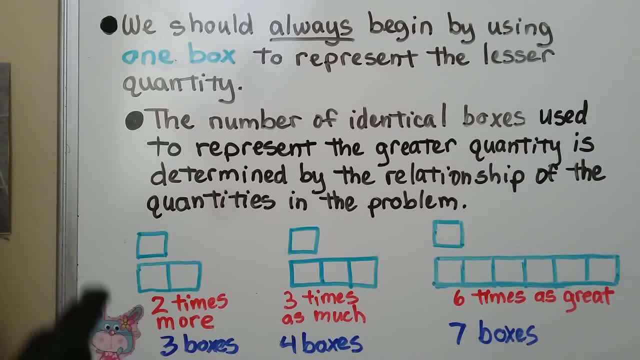 words in the word problem. If it says 2 times more, we're going to draw our one box for the lesser quantity and then two boxes for the 2 times more. That's three boxes in all. If it says three times as much, we draw one box for the lesser. 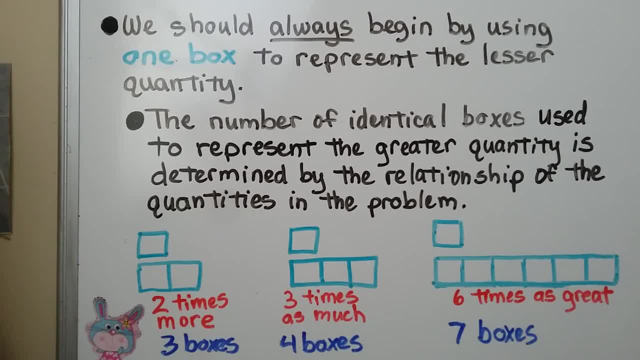 quantity and three boxes for the three times as much, which is four boxes in all. If it says this is six times as great, then we draw one box for the lesser quantity and then two boxes for the two times, then six boxes for six times is great. That's seven boxes in all. 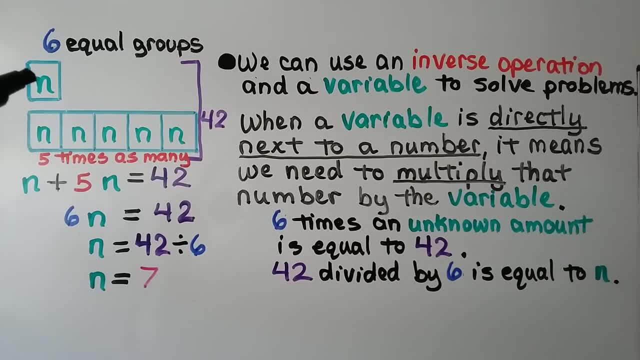 Here our bar model shows one box for the lesser amount, and then there were five times as many. so there are five boxes drawn here, That's six equal groups, and we can use an inverse operation and a variable to solve problems. We say that this is n, so this is five n's. 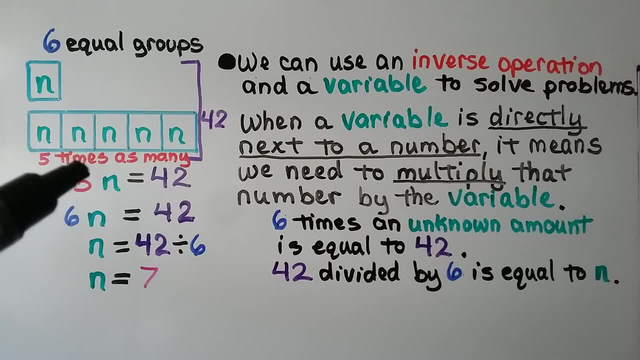 That means we have an n plus five more n's and we can see it's equal to 42.. There's a bracket with the 42 showing their total And when a variable is directly next to a number, it means we need to multiply that number. 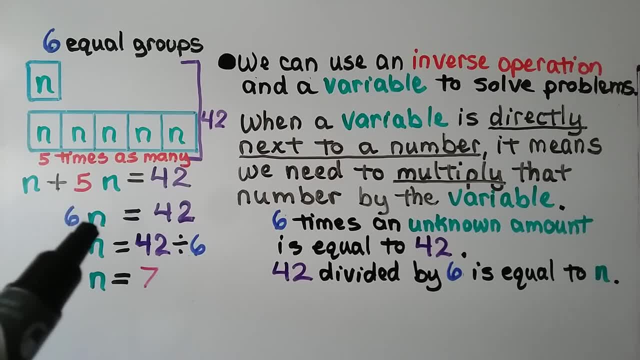 by the variable. This is six times an unknown amount because, remember, a variable takes the place of an unknown amount and it's equal to 42.. We can use the inverse operation and find 42 divided by six to equal n. 42 divided by six is seven. That means n is equal to seven. This one n is equal to seven. 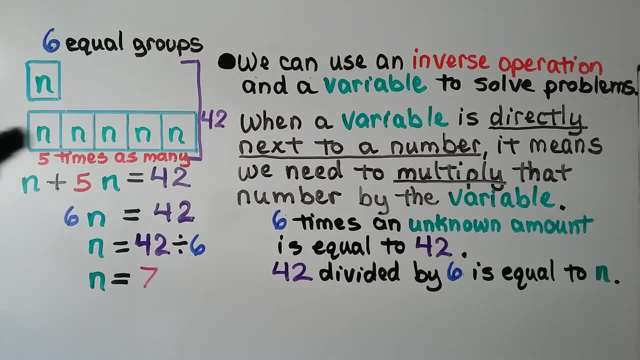 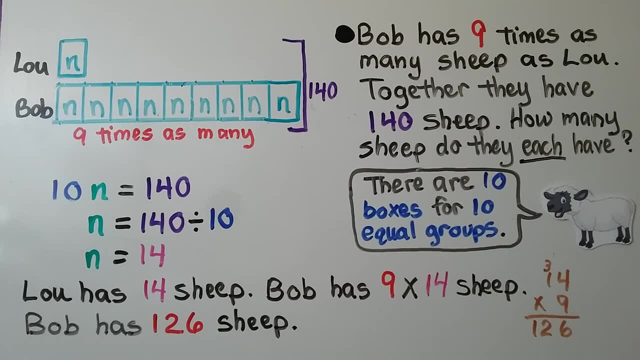 This is five times seven, so these would be 35.. Bob has nine times as many sheep as little. Together they have 140 sheep. How many sheep do they each have? So because Bob has nine times more than Lou, nine times as many, we know Lou has the lesser amount. 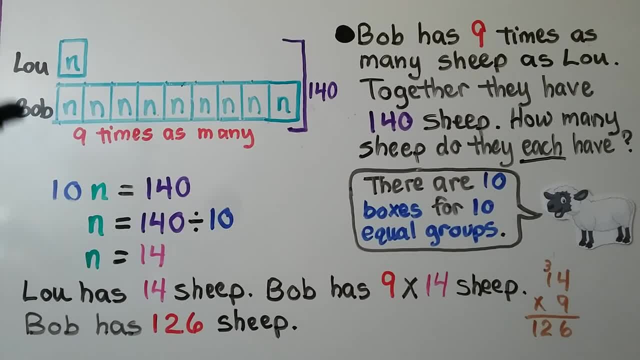 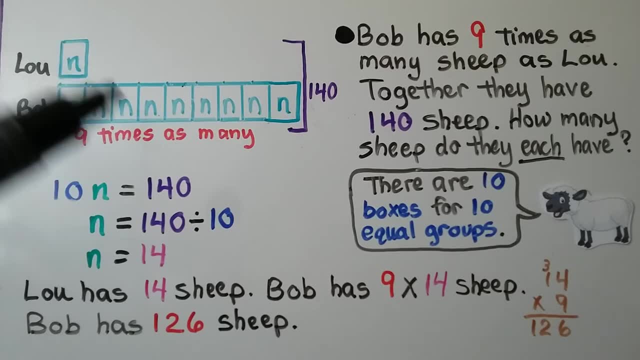 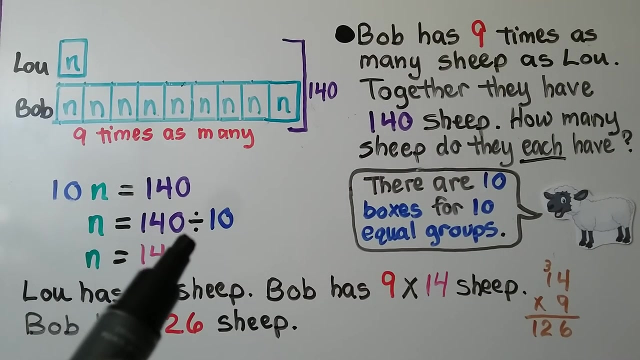 We make one box for Lou, and Bob has nine times as many, so we make nine boxes for Bob. There are ten boxes for ten equal groups. all together That means we have ten times some number. n is equal to 140.. We can use the inverse operation of 140 divided by 10 will equal the n. 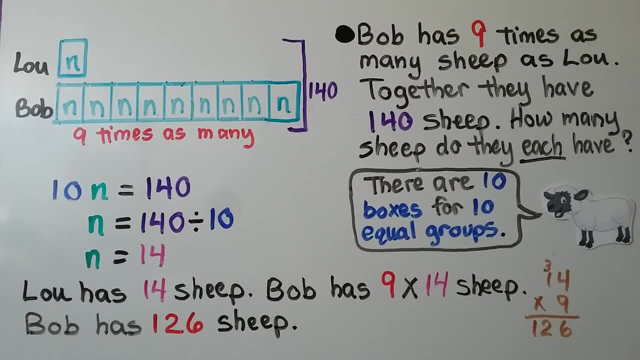 140 divided by 10 is 14.. That means n is equal to 14.. So we know Lou has 14 sheep and Bob has nine times as many We do. 14 times 9 is equal to 126, so Bob has. 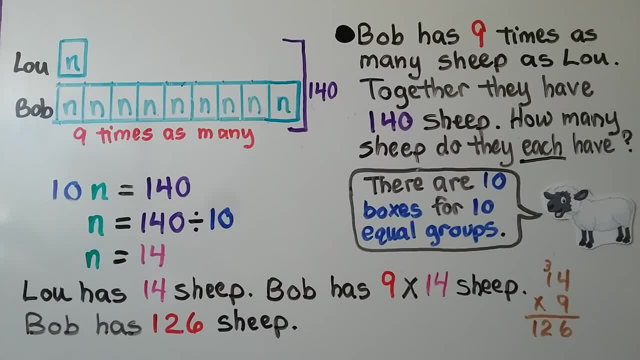 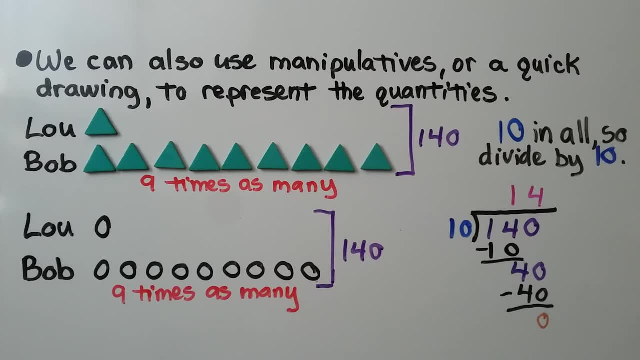 126 sheep. We can also use manipulatives or a quick drawing to represent the quantities. We can give one counter for Lou and nine counters for Bob, because he has nine times as many. We can draw a circle for Lou and nine circles for Bob, because he has nine times as many. 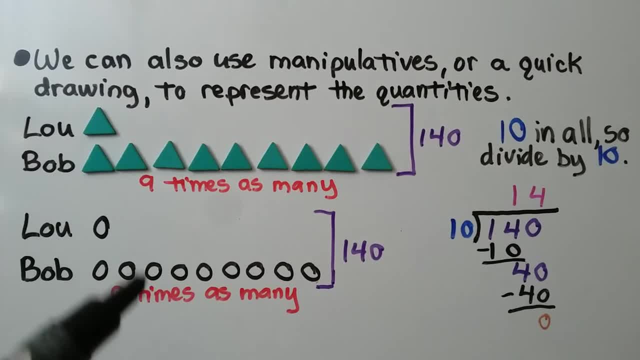 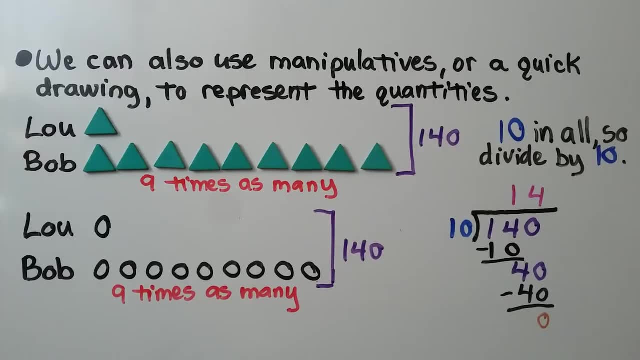 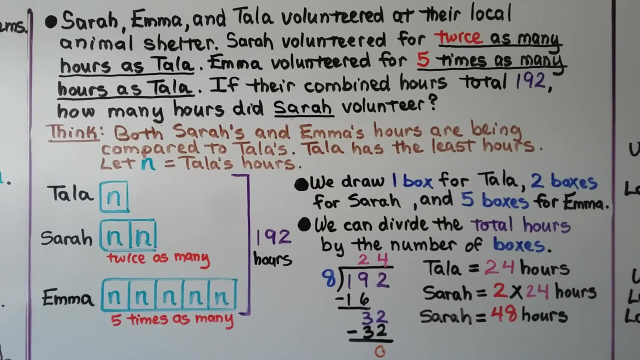 There's ten counters in all, or ten circles in all, so we're going to divide 140 by 126.. by 10.. Sarah, Emma and Tala volunteered at their local animal shelter. Sarah volunteered for twice as many hours as Tala. Emma volunteered for five times as many hours as Tala. If their combined 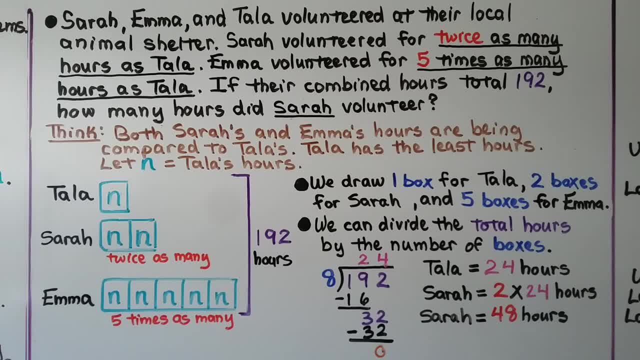 hours total 192,. how many hours did Sarah volunteer? So we're trying to find Sarah's volunteer hours, But do you notice that both Sarah and Emma's hours are being compared to Tala's And Tala has the least hours, Sarah's twice as many as her and Emma's five times as? 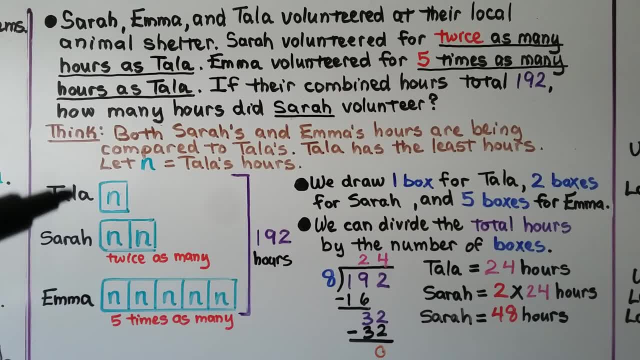 many as her. So we know Tala has the least hours. We're going to let n equal Tala's hours. We draw one box for Tala. Sarah is twice as many. So we draw two boxes for Sarah, And Emma is five. 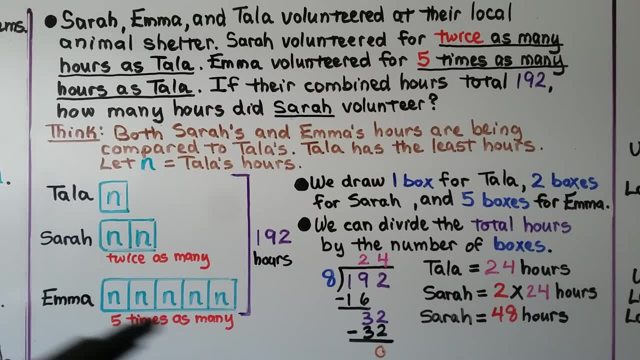 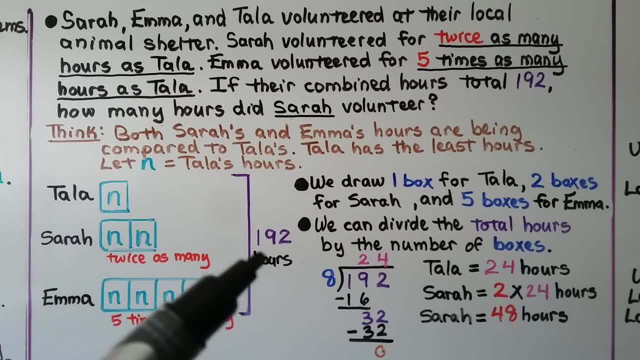 times as many And Tala is twice as many as Tala. So we draw five boxes for Emma, We have our bracket with our 192 for the total combined hours And we can divide the total hours by the number of boxes We've got. 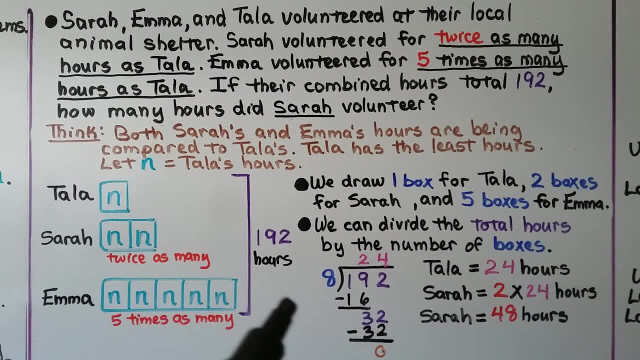 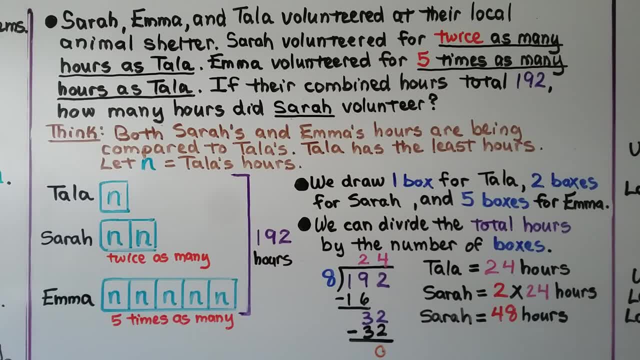 And we can divide the total hours by the number of boxes. And we can divide the total hours by the number of boxes. Sarah volunteered for 48 hours. Now you may be asking yourself: why did we need Emma? Emma wasn't even part of the problem, you would think, but she was part of the problem. 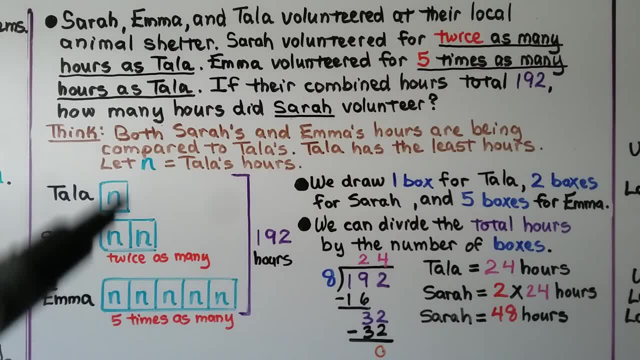 We needed Emma's five boxes to know that we needed to divide 192 by 8. If we only divided by Sarah's two boxes and Tala's one, we wouldn't have gotten the right answer for Tala's hours. We needed all of their boxes so we could represent all the equal groups as 8 equal groups. 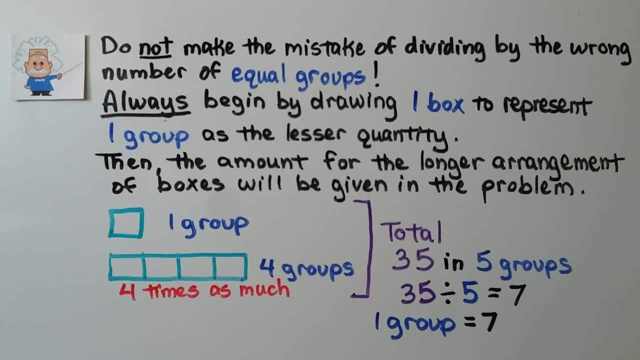 Do not make the mistake of dividing by the wrong number of equal groups. Always begin by drawing one box to represent that one group as the lesser quantity, then the amount for the longer order. The total number of groups we will have is 4.. 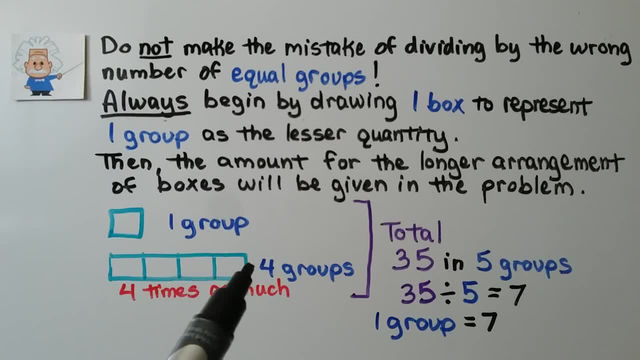 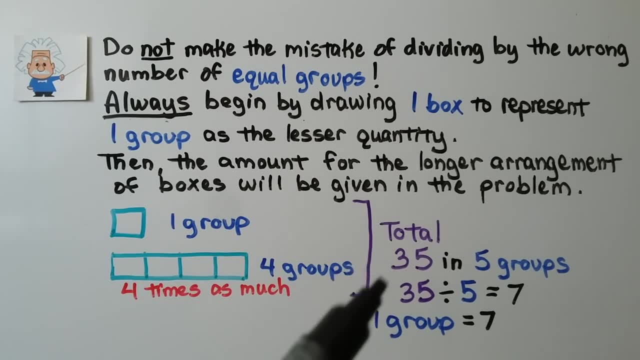 The area down the left is where the problem ends. Now that we have a total of 3.5, we need to divide this by 3.5. Let's look at our problem to calculate the total number of groups in the question. 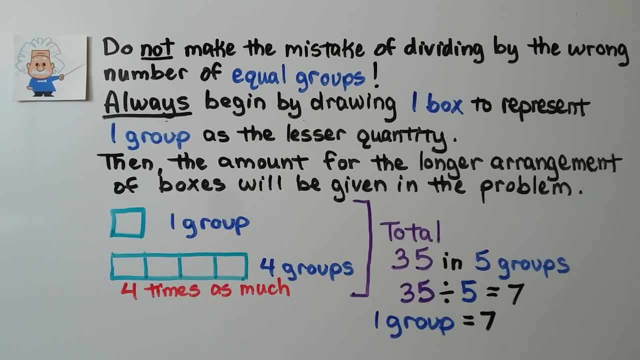 Both 5 and 3 are equal, so we know that the value of 3.5 is 35.. The value of 5 and 5 is the number of groups in the question. The answer to this problem is nochmal: By dividing on the second line, we get the step number to 4.4. 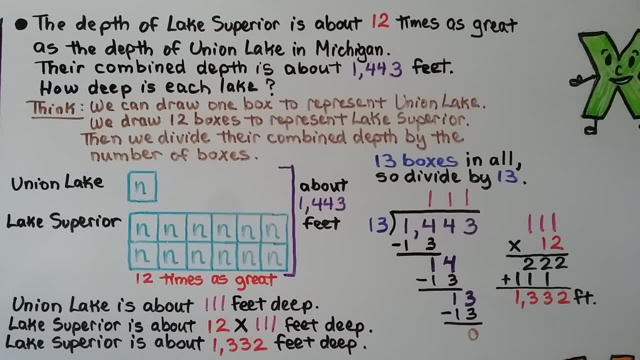 The answer to this problem is again the same as the first line, but the step number is bigger than the first line of Union Lake in Michigan. The combined depth is about 1,443 feet. So how deep is each lake? So we think we can draw one box to represent Union Lake, because it's not as deep. It's the 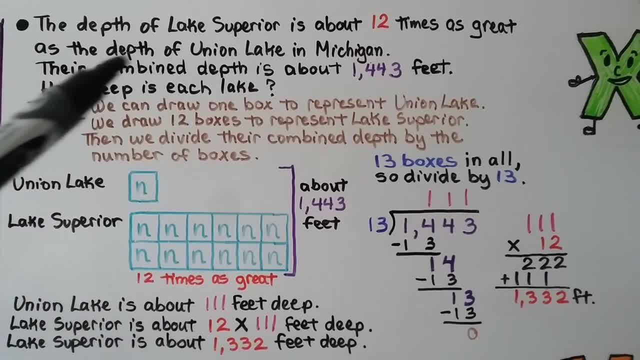 lesser amount. Lake Superior is 12 times as great as that. So we know Union Lake is our lesser amount. We're going to make one box. We draw 12 boxes to represent Lake Superior, and we can even stack them like this in an array, as long as we have 12 of them. Then we divide their combined. 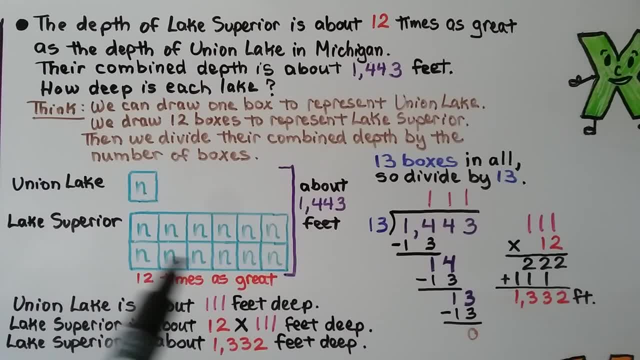 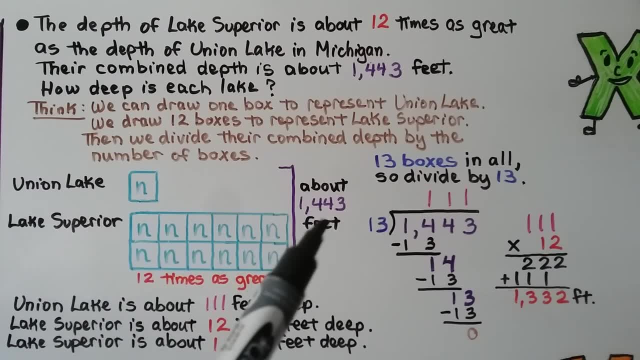 depth, the 1,443, by the number of boxes. If we have 12 here and one here, that's 13.. We have 13 boxes in all, So we're going to divide the combined depth by 13 and we do. 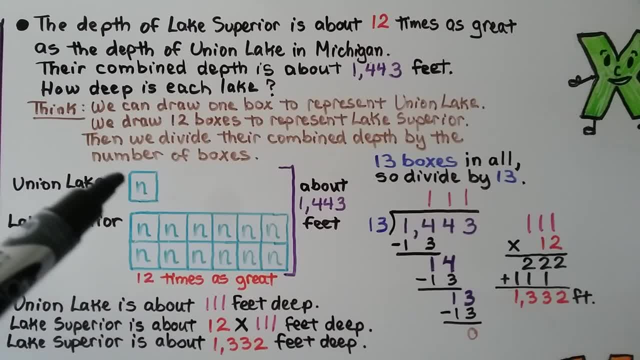 And we get 111.. That means Union Lake is about 111 feet deep And Lake Superior is 12 times as great of a depth. So that's 12 times 111.. Do a little multiplication on the side and see that that would be 1,332 feet. So that's the depth of Lake Superior. 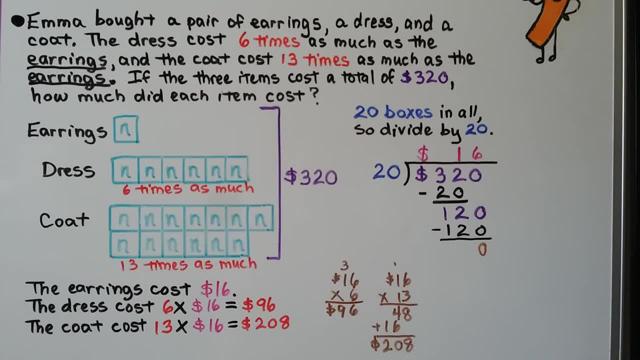 Emma bought a pair of earrings, a dress and a coat. The dress costs six times as much as the earrings And the coat costs 13 times as much as the earrings. If the three items cost a total of $320,, how much did each item cost? So, if you noticed, the dress and the coat are being compared. 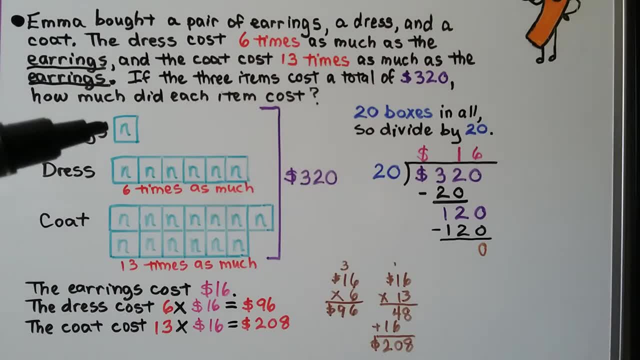 to the earrings. We know the earrings would be the lesser amount, So that's going to be our one box, our N. The dress was 6 times as much as the earrings, and so we're going to have 6 times 1, that's 6. 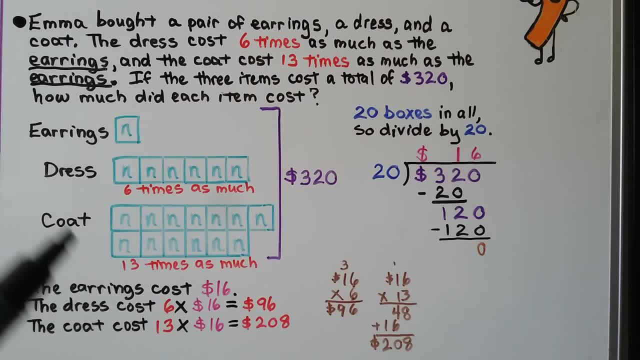 boxes And the coat was 13 times as much as the earrings. So we're going to have 13 ames 1, that's 13 boxes, and we can stack them like this, with a seven and then a six for the 13.. 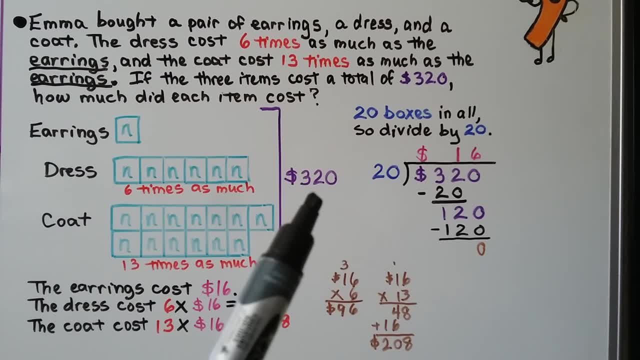 We draw our bracket with our $320 for the total cost And we count the boxes. We have 13 and six, That's 19 and one more is 20.. So 20.. We have 20 boxes in all, so we're going to divide by 20.. $320 divided by 20 is $16.. 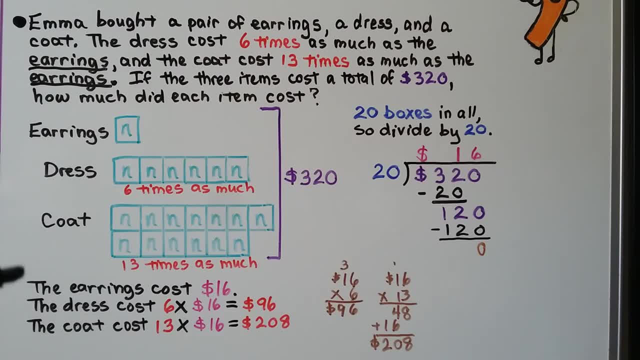 So we know the cost of the earrings. they're $16.. And the dress costs six times the price of the earrings. so we know it's six times $16. We do a little multiplication and see it's $96.. The coat costs 13 times $16.. We do a little multiplication and see that it's. 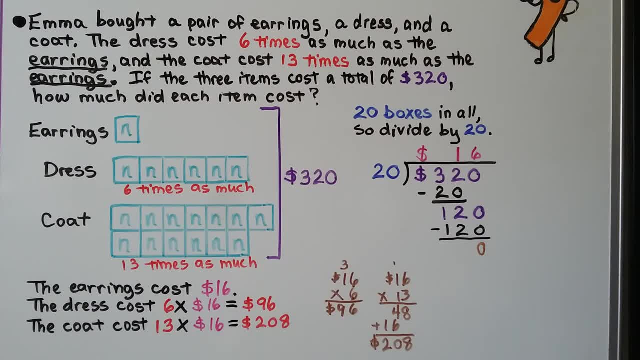 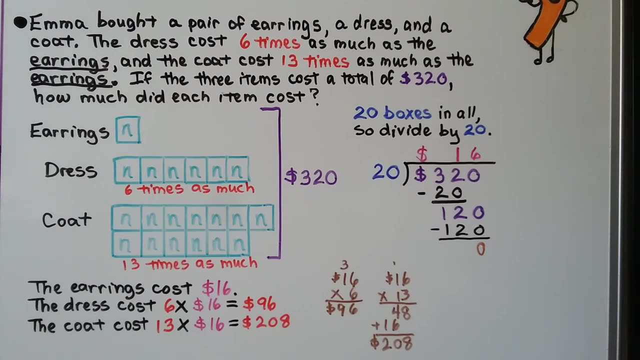 $208.. It's very important to see what we were comparing them to. Both the dress and the coat were being compared to the earrings as more, six times more or 13 times more, So we knew the earrings were the lesser amount and that was going to be our one box. 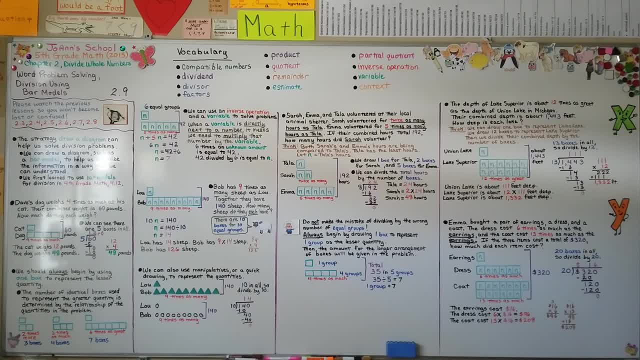 So the most important thing you need to remember is to not make the mistake of dividing by the wrong number of equal groups. We should always begin by using one box to represent the lesser quantity. Then the amount for the longer arrangement of boxes will be given in the 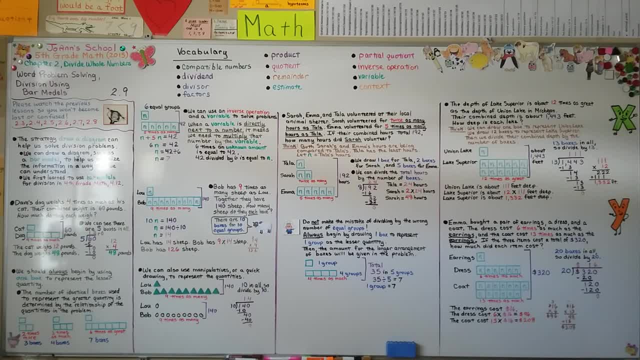 problem. Okay, we're going to move on to chapter three. We're going to be talking about adding and subtracting decimals. I hope I'll see you there and stay safe, stay strong, Bye. 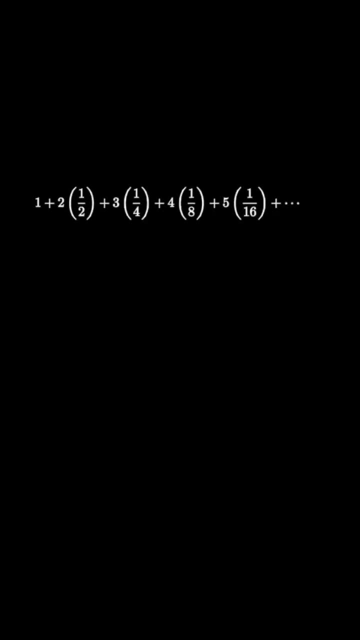 Here's an interesting infinite sum: 1 plus 2 times a half, plus 3 times a quarter, plus 4 times an eighth, and so on. Do you know how to find the sum of this infinite series? What if I showed you this geometric picture? Would this help you figure it out? 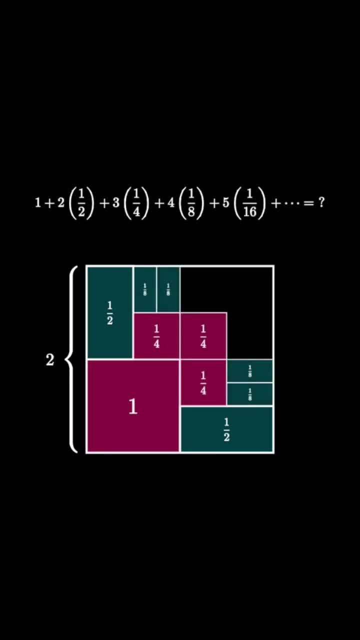 Can you figure out the sum now? Let me know in the comments. 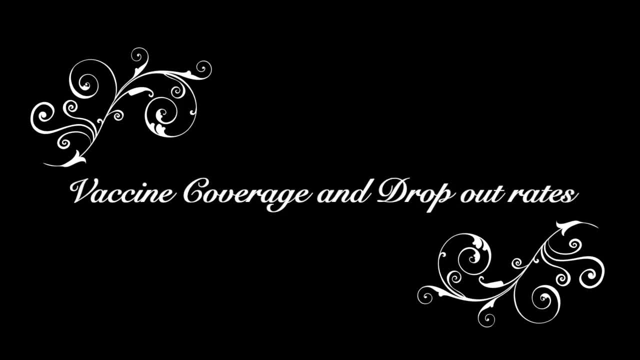 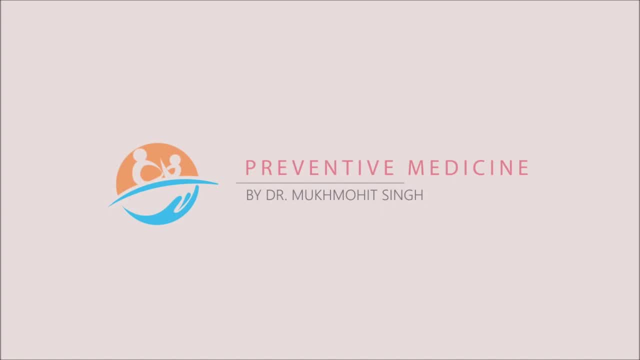 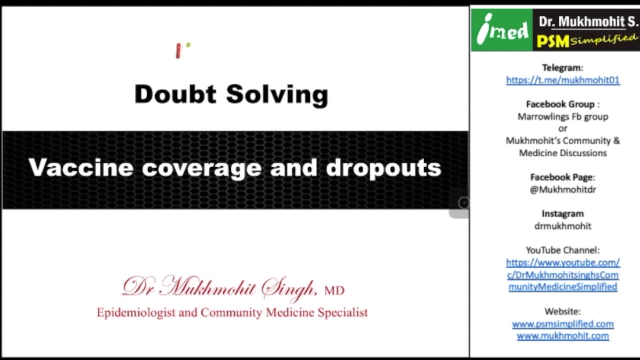 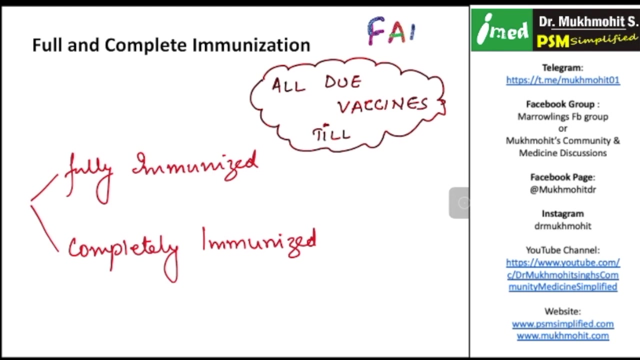 Hello and a very warm welcome to all of you today, the 10th of March 2021.. We are going to have another short doubt-solving session on vaccine coverage and dropout rates. So before I proceed any further, let us have a quick discussion on a very frequently asked doubt, that is, pad. that what? 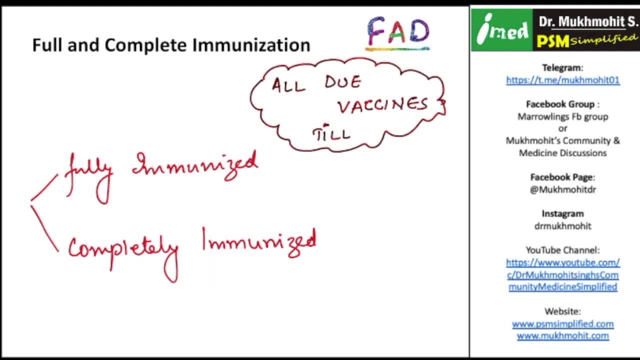 do we mean by a fully immunized child and what is a completely immunized child? Please remember that what is a fully immunized child? Fully immunized child is a child who has received all due vaccine, who has received all due vaccine till one year of age, So fully immunized till one year of age. and